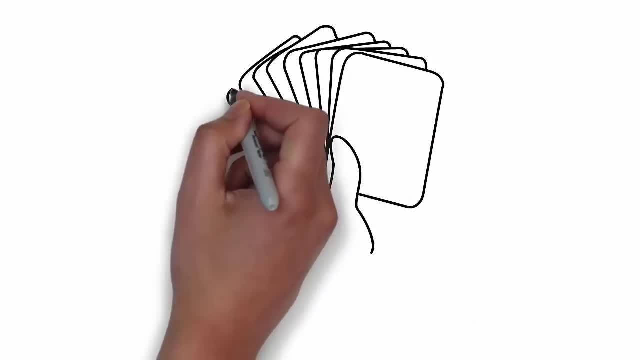 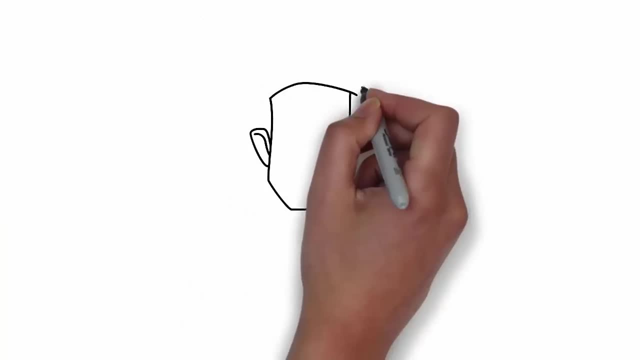 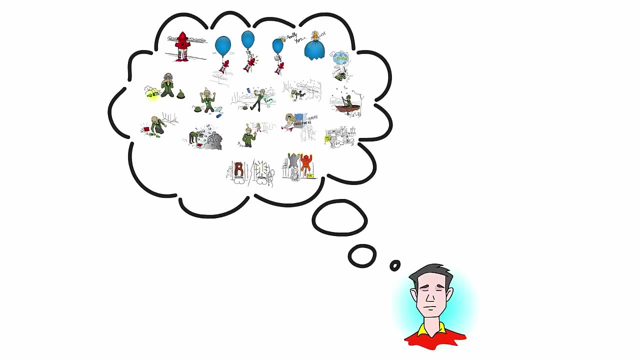 When a memory expert memorizes playing cards or the first thousand decimals of pi, they use mental imagery techniques. In this series of videos, you are going to memorize the first 20 elements of the periodic table by doing what the experts do. I'll tell you exactly what's picture in your mind. 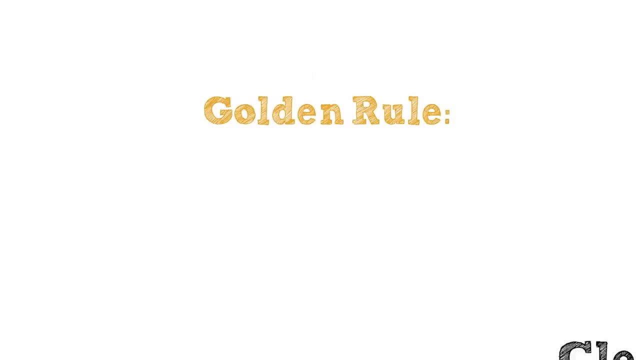 and I'll even draw it for you too. Focus on seeing each picture in your head, and you'll be amazed at how easily you can recall everything. Let's get into it. We'll begin by picturing a typical poster or chart of the periodic table. There are many small colorful squares, each with a name number. 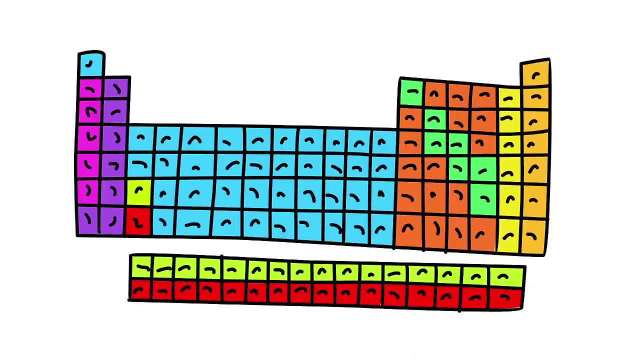 and symbol of an element, and together they create a large irregular shape. This image will act as an anchor in your memory, holding down the chain of images which link together all the elements. Now we'll take that colorful poster and attach it to the first element. Picture that poster of the. 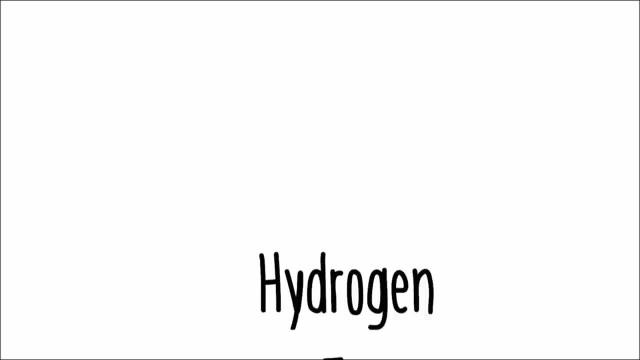 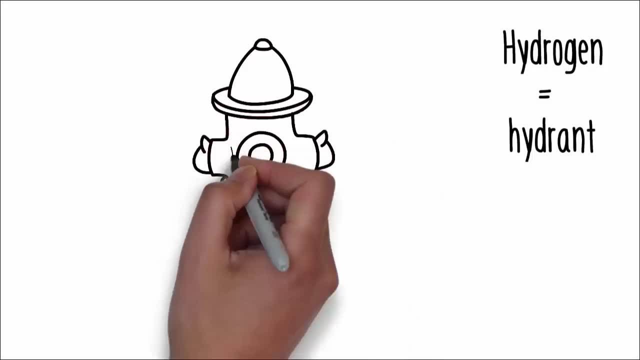 periodic table and imagine it's wrapped around a water hydrant. Why a water hydrant? The first element in the periodic table is hydrogen. Hydrogen sounds similar to hydrant and that's how you'll be reminded of it. Picture a water hydrant. 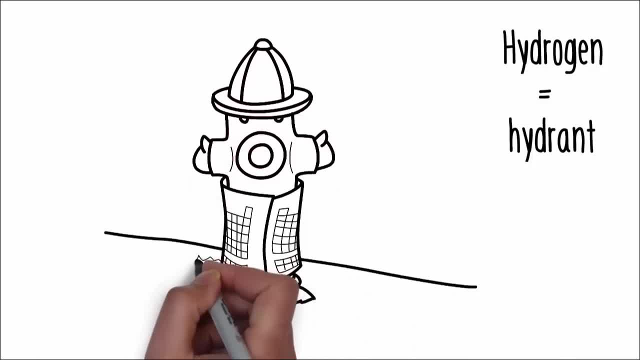 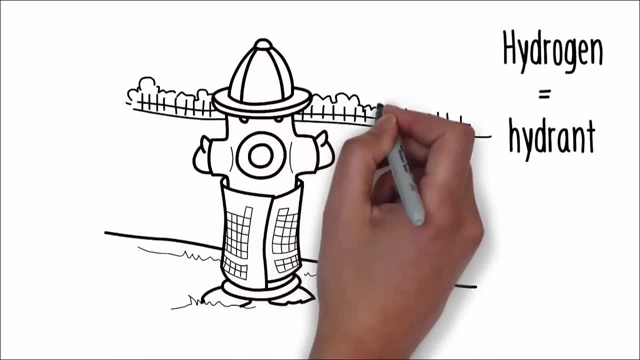 you see on the sidewalk. It's short, stubby red and looks strong. The hydrant is like a little man with a small hat on top and stubby arms sticking out the side. Imagine that hydrant with the chart of the periodic table wrapped around it. When you think of the chart of the periodic table, you'll 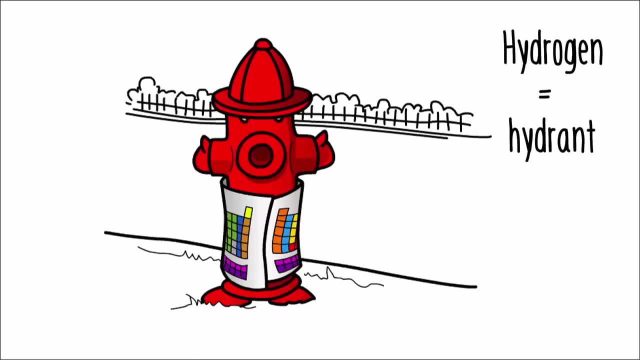 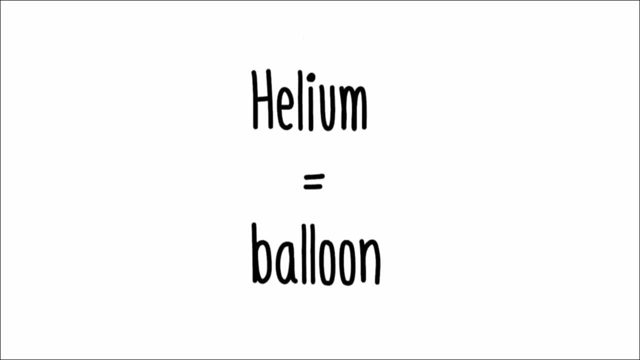 picture it wrapped around a water hydrant, Because hydrant sounds similar to hydrogen. you'll know the first element in the table is hydrogen. The second element is helium. If you're like me, when you think of helium you automatically think of a helium balloon. When 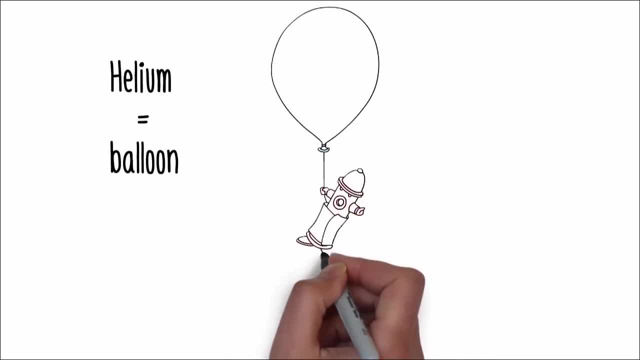 you let it go. it's the type that floats up into the sky. Now imagine an enormous helium balloon. Make it the size of a car and picture it attached to the water hydrant. Because the helium balloon is so big and has so much lifting power, it starts to lift the water hydrant up off the sidewalk. 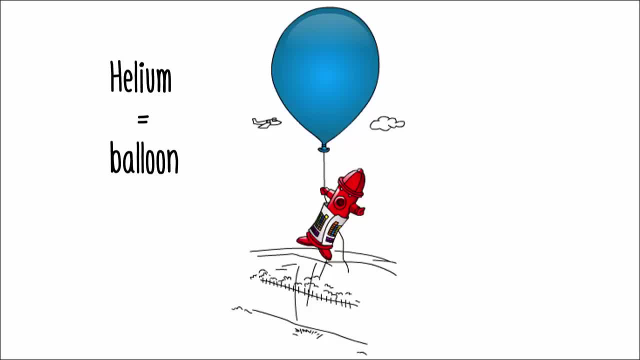 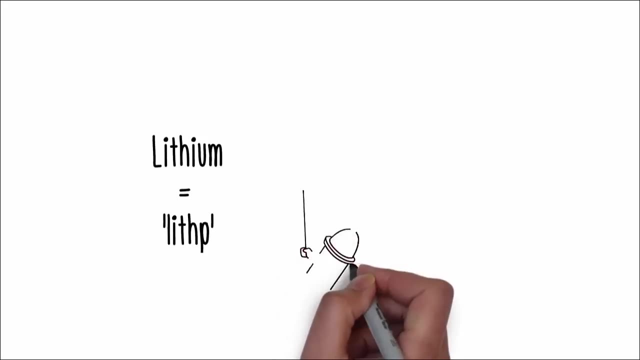 Together. they slowly float up into the air and away into the sky. Now, when you visualize the hydrant, you'll know. the second element is helium. The third element is lithium. Lithium sounds a bit like lisp. People that have a lisp, a type of speech impediment, aren't able to pronounce lisp. 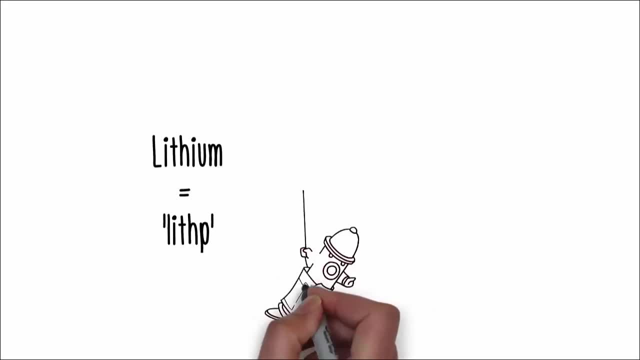 and say lisp. Let's pretend the large helium balloon has a lisp. It also has a small hole in it, causing the balloon to slowly deflate. Usually a balloon with a hole in it will make a slow sss sound, But because this balloon has a lisp or lisp, it makes a fff sound. 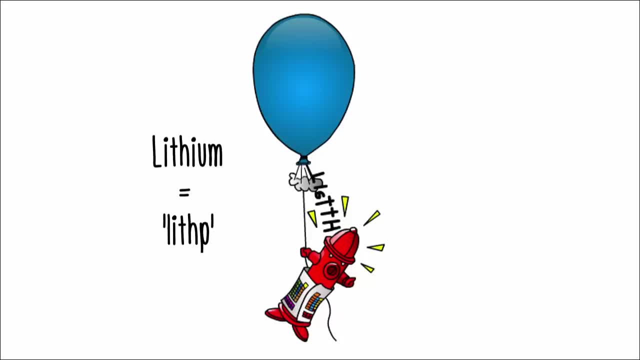 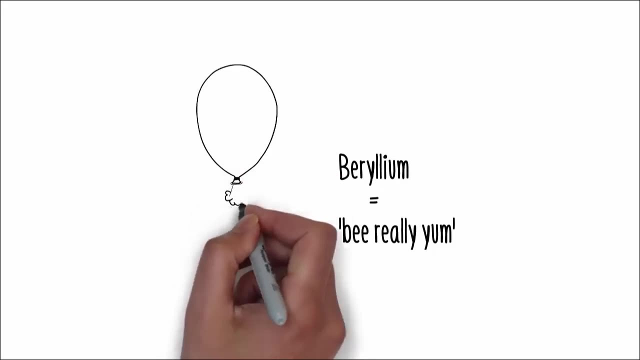 Visualize the large balloon slowly deflating, making a th sound. Now, when you think of the balloon's lisp, you'll be reminded of the third element, lithium. The fourth element is beryllium. If you say beryllium slowly, it sounds like bee really. yum. Picture: you're a slowly deflating 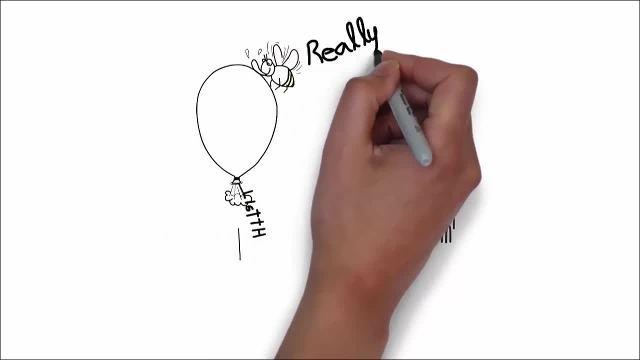 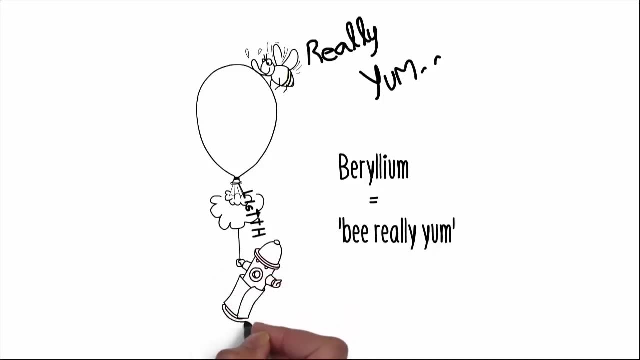 balloon. Now imagine an enormous bumblebee lands on the balloon. The bee is the size of a football. loudly, The bee licks the balloon to have a taste and says: hmm, really yum, It really likes the taste of the balloon. When you picture the bee licking the balloon you'll think: bee, really yum and be. 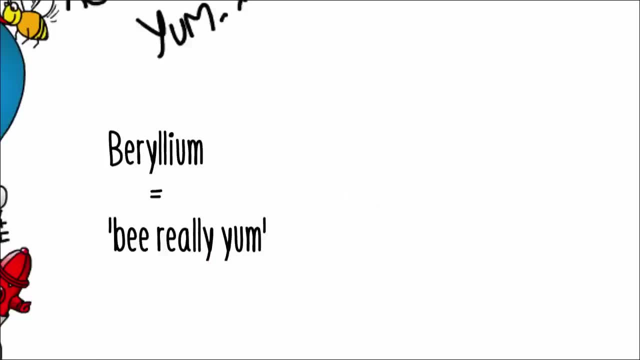 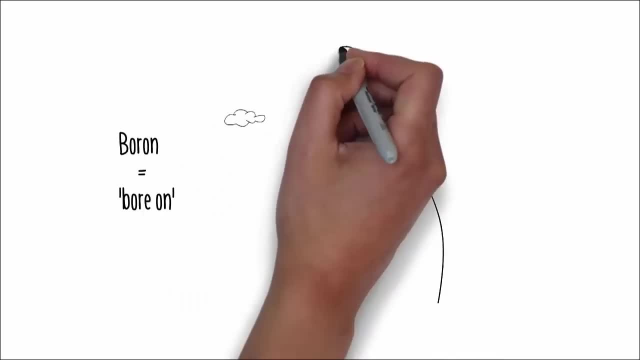 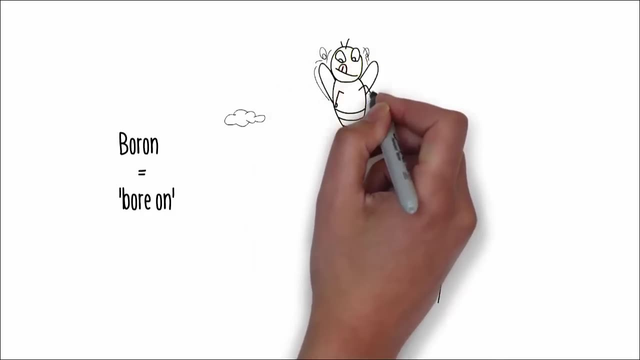 reminded of the fourth element, beryllium. The fifth element is boron. We can break up the word boron into bore, and on The word bore, b-o-r-e can mean to drill a hole. Picture now: the bee, after it uses its stinger, pierces the balloon and starts to spin around in a drilling motion. The bee has 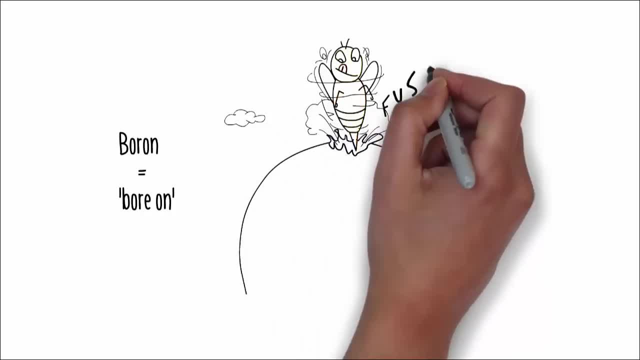 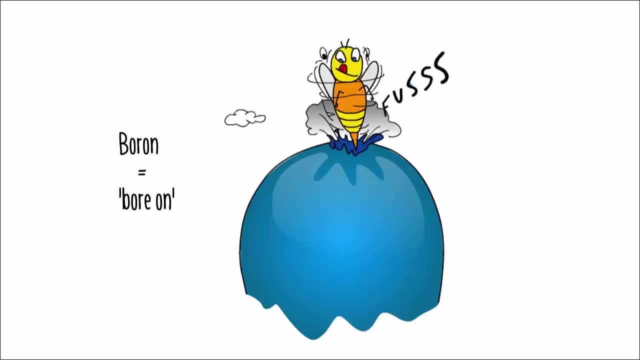 landed on the balloon, tasted it and now it's started to bore on the balloon. When you picture the bee begin to bore on the balloon, you'll remember the fifth element, boron. All right, that's the first five elements of the periodic table. I'm sure you can easily remember them. but 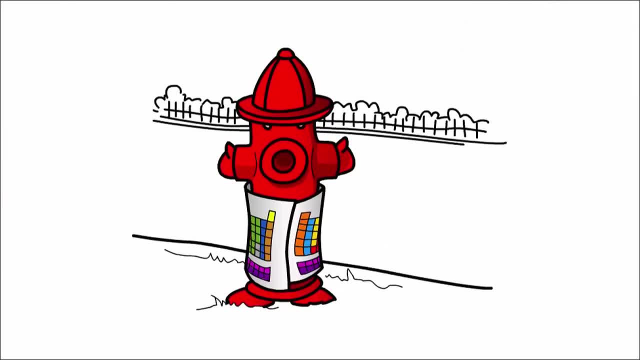 quickly revise your memory story now by replaying it and watching it in your mind. Picture a poster of the periodic table. The poster of the periodic table is wrapped around a hydrant which reminds you of hydrogen. The hydrant starts to float up into the sky because it's got a huge helium balloon. 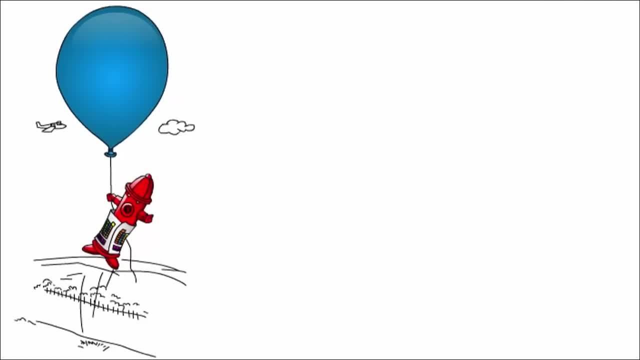 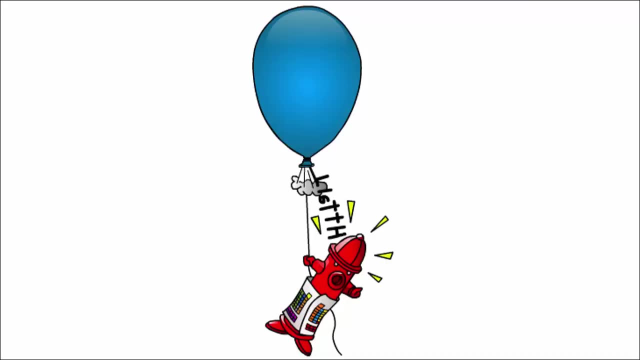 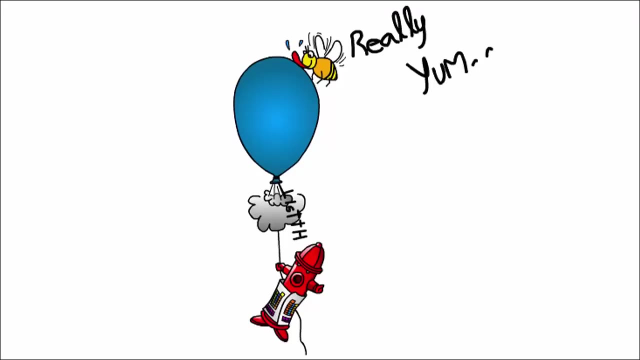 attached to it, reminding you of helium. When it gets high up in the sky, the balloon starts to slowly deflate and makes a th sound because it has a lithp giving you lithium. Then you see a huge bumblebee land on the balloon. lick it and declare it's really yum, Bee, really yum- beryllium.